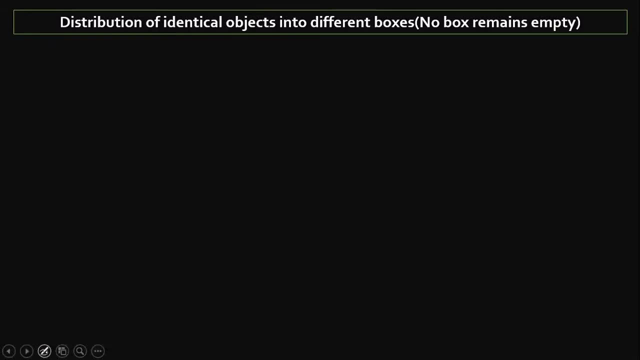 Hello friends, in the last video class, the last lesson, what we have discussed is the number of ways, what we have discussed. once I will write the number of ways of distributing, the number of ways of distributing n identical objects. the number of ways of distributing n identical objects. 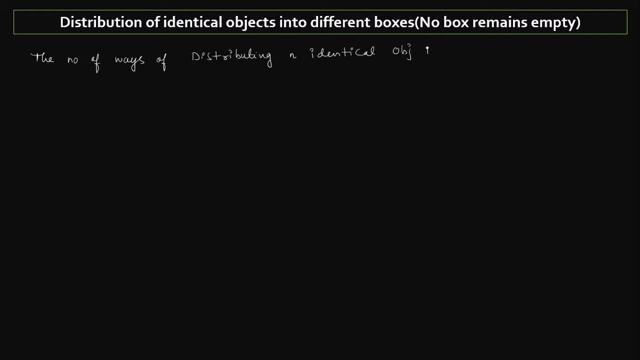 n identical objects into r distinct boxes, r distinct boxes. that is same as without any restriction, without any restriction, without any restriction. What is the meaning of this? without any restriction, The meaning is this: the box may be empty, may not be empty. 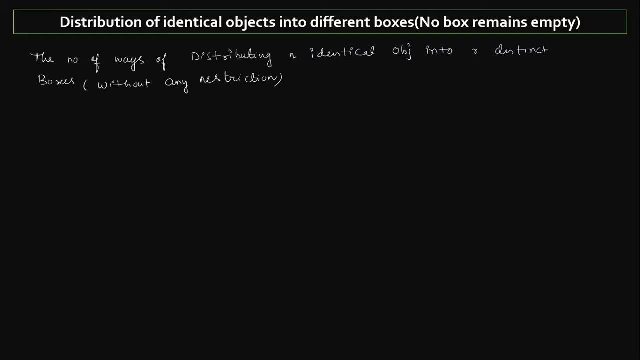 So each and every box contains any number of objects. There is no restriction on that. A box may be empty, also right. So the number of ways of distributing n identical objects into r distinct boxes without any restriction is what Is same as the number of it is same as the number of non negative, non negative integral solutions. 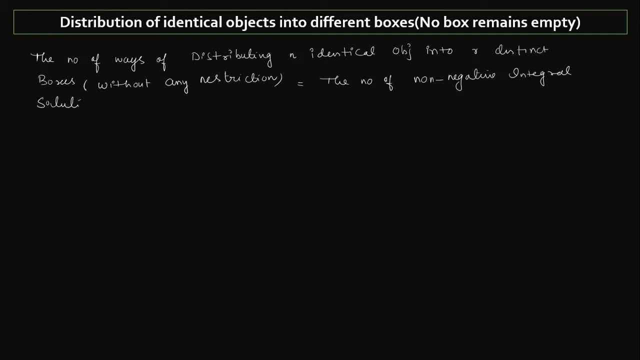 So the number of non negative integral solutions of the linear equation. what is that linear equation? x1 plus x2 plus x3 plus up to so on. xr is equals to n. is what What we have written? n plus r minus 1, cr minus 1.. So this we have seen in the last class. So if you did not watch this, go to that video and watch first before seeing this. 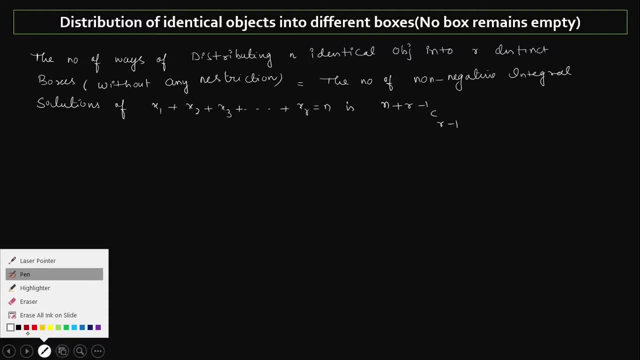 So this we have seen in the last class. So if you did not watch this, go to that video and watch first before seeing this. watching this, okay, right, so here. what is r in this? what is r in this? r is number of boxes. 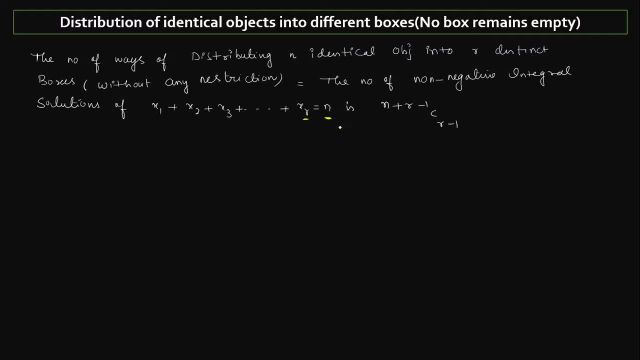 and what is? a number of objects. the right hand side number. what you are seeing in the equation, it is nothing but the number of the number of objects. how many objects, how many identical objects given to you? and what is this r represent? this r represent number of boxes. 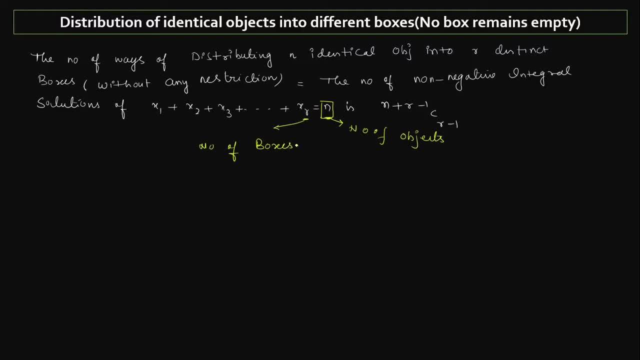 this r represent number of boxes. okay, now here. what we are going to do is now little bit changes in this. what we are going to do is, let us say: um, for example, the second condition means the second derivation. okay, in a different situation, that is the number of. for example, if i want the number of, 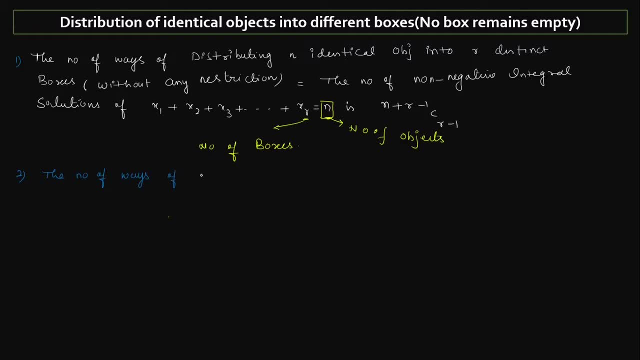 number of ways of distributing, the number of ways of distributing n identical objects, n identical objects, same, into r distinct boxes, r distinct boxes. but here the condition is no box remains empty. That is the restriction we have in this: The number of ways of distributing n identical objects. there also n identical objects. we. 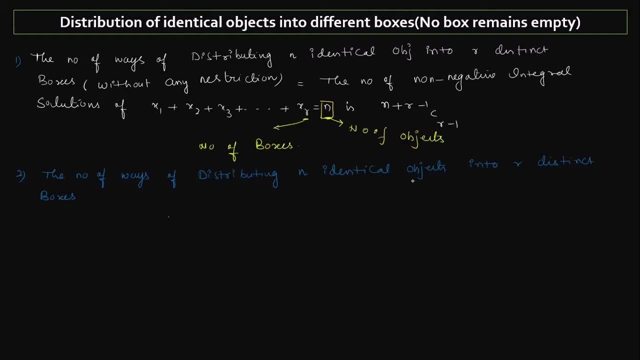 are distributing here also n identical objects. we are distributing there also. we have r distinct boxes. here also we have r distinct boxes. but here the condition is: here we have no condition, no restriction on this, but here we have a restriction, so that no. 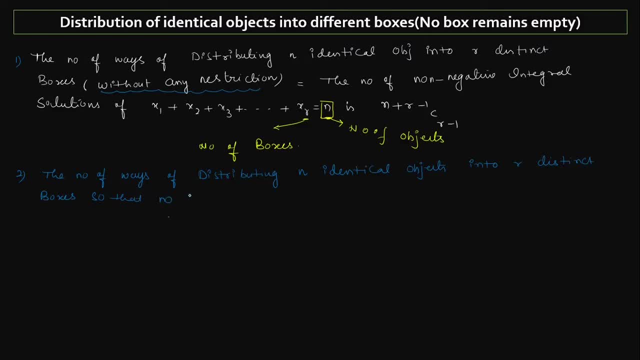 box remains empty, So that no box remains empty empty. So what is the meaning of this? No box remaining empty means each and every box must have at least one object. Each and every box must have at least one object in the box. 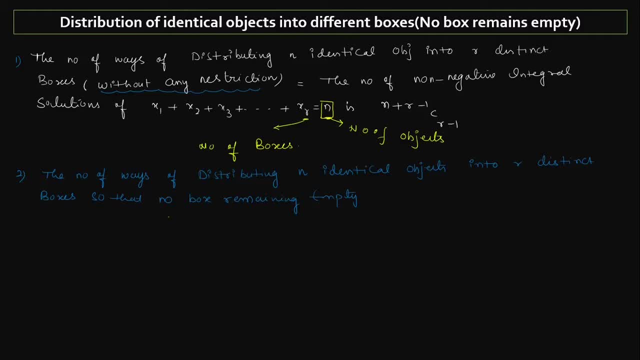 So how we will do this? The same way, how we done the first derivation, the first derivation, how we did, in the same way we can do, but instead of that, what we are going to do, we will take the help of this, we will take the help of this to derive this property. Actually, the result is: 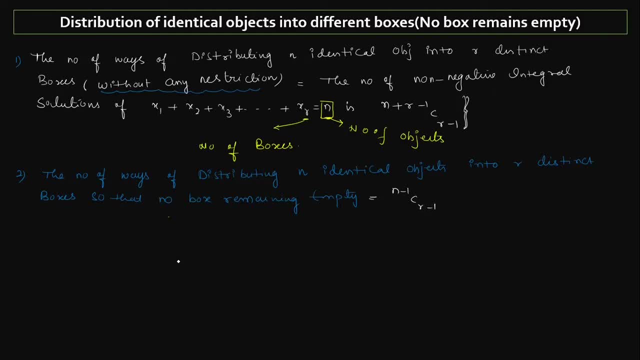 this: n minus 1, c? r minus 1 is the result. Number of ways of distributing n identical objects into r distinct boxes so that no box remains empty, is what The number of ways is what? n minus 1, c? r. 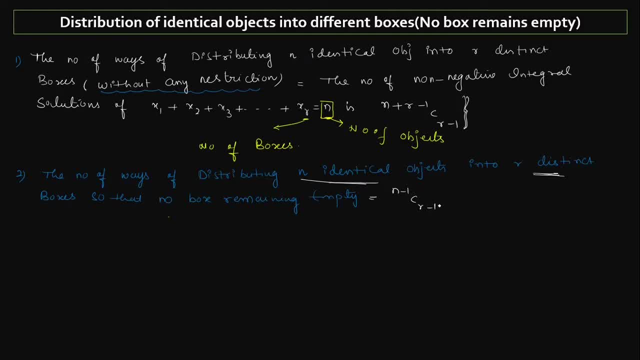 minus 1.. So how we will get this: n minus 1, c, r minus 1? With the help of this we will get the help of the property, or with the help of the derivation, what we have already. Let us see now. 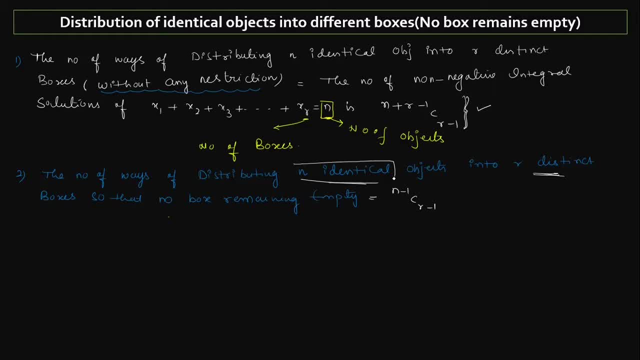 Now what is the work we have to do Here? we have to distribute this n identical objects into what r distinct boxes. Now let us say: here we have the first box, second box, third box, we have r distinct boxes. Let us suppose I am placing x1 objects in the first box, x2 objects in the second. 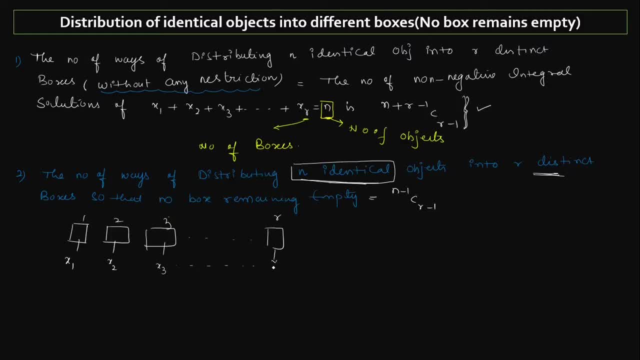 box x3, objects in the third box. Like that I am putting xr objects. number of objects we are placing in the rth box is xr. So if you add all these variables- number of objects in the first box plus number of objects in the second box, plus number of objects in the third box, up to so on- 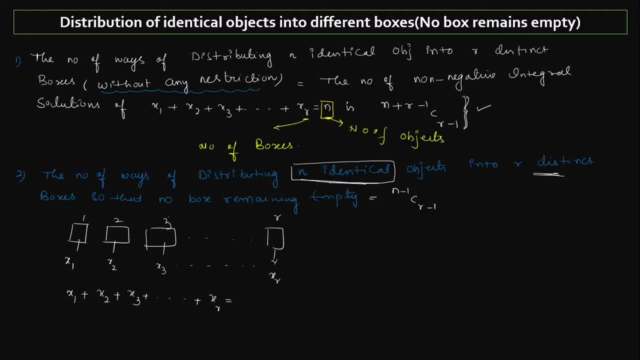 number of objects in the rth box must be equal to total number of objects. right, Because of we are distributing all the identical objects into these r boxes. So therefore x1, figure 3, x2 plus x3, plus up to so on. xr must be equals to n. but what is the condition? here? no box remains. 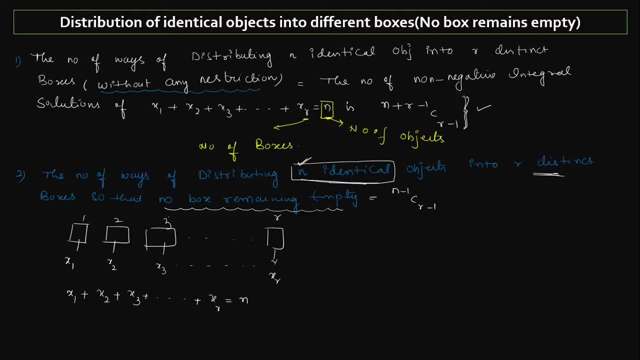 empty. no box remains empty means first box holds at least one object. so therefore, the value of x1 is minimum one. the value of x1 is how much minimum one? similarly, what is the value of x2 is also minimum one. at least one object should be there in the second box also, at least one object should be. 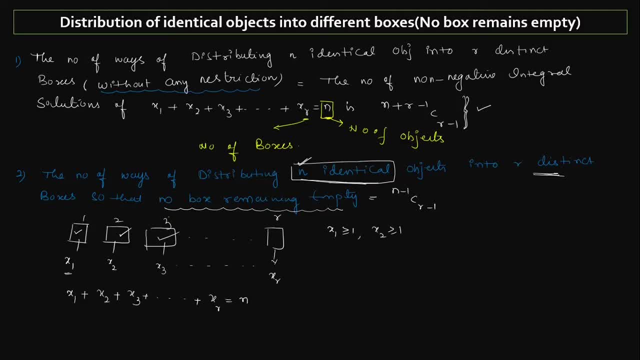 there in the third box also. each and every box must hold, at least, must have at least one object in that. okay. so therefore, each xi, each xi must be greater than or equal to one. okay, each xi greater than or equal to one, for what i is equal to one, as well as two, as well as three, up to so on r. 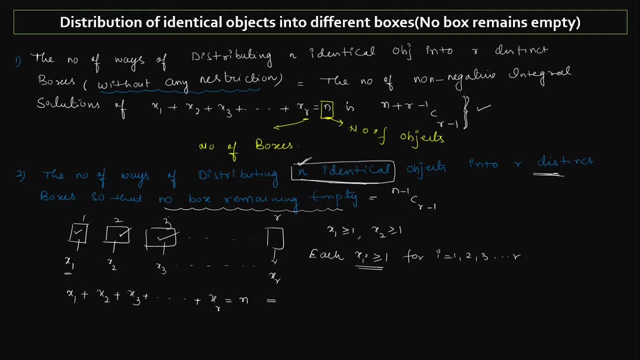 so what we are going to do here, this equation, i am going to change now x 1 from this. we will write x 1 minus 1 in place of x 2. i will write x 2 minus 1 plus up to so on for each. 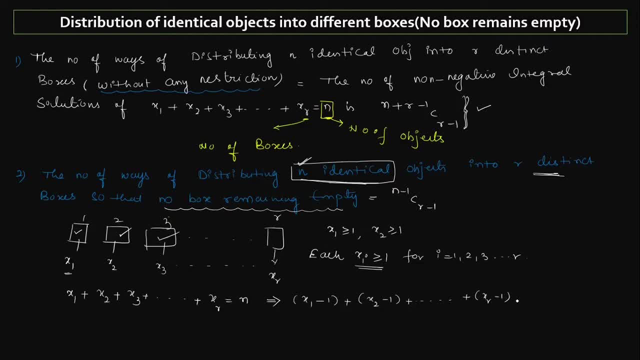 variable. i am subtracting 1 for each variable. i am subtracting 1, so therefore total: how much we subtracted: minus 1 minus 1. minus 1 r times means minus r. we subtracted that. okay, so r is subtracted from the left hand side, so we have to subtract from the right hand side also: n minus r. sorry. 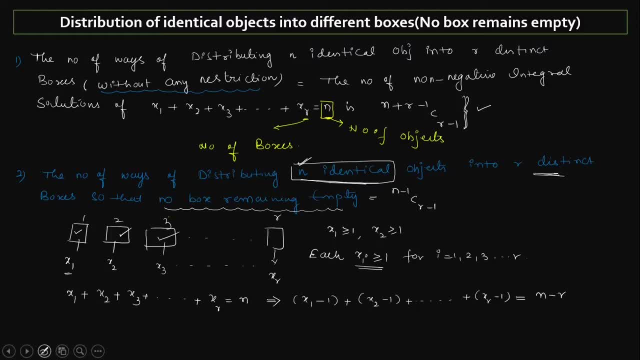 now what i am going to do here. we are going to write in place of this x 1 minus 1, in place of this x 1 minus 1, i give a new symbol for that say: that is capital x 1. okay, here capital x 1 is x 1 minus 1 and x 2 minus 1. i will suppose. 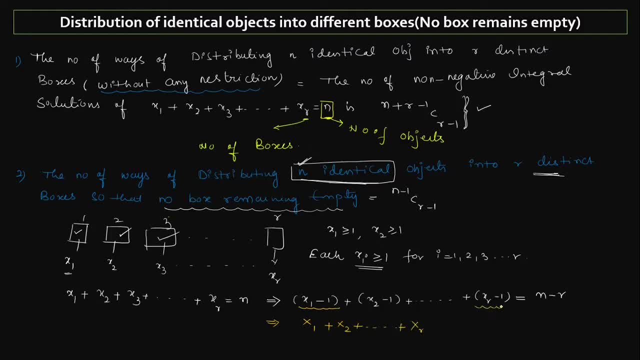 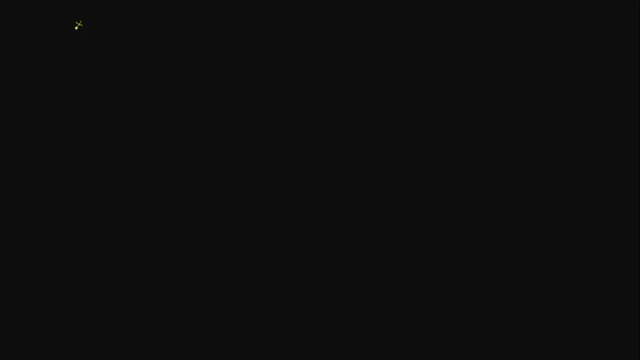 as capital x 2, plus up to so on capital x r. this i am supposing as capital xr, which is equal to n minus r. okay, now let's go to the next slide. here i'll write so what i got in the last slide: x 1. plus x 2 plus. similarly, if you want, you can write one more x3 plus x 2 as x 2 up to x 1. you can write one more: x 3 plus x 3 plus x 2, x 2, a value of x 1 minus x 2 and the other things that we have seen in the previous volume. 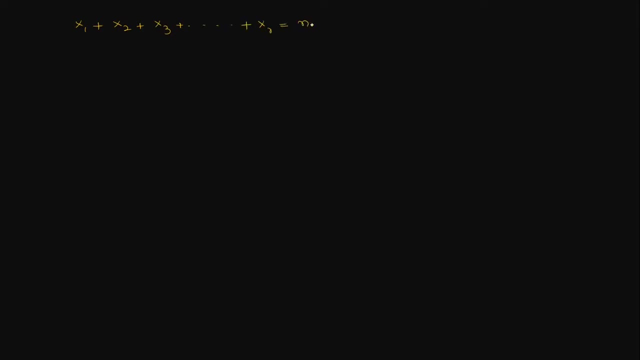 up to so on. xr is equals to what do we have here? n minus r. Now in this, what is x1?? x1 is x1 minus 1, which is greater than or equal to 0, already we know that. So x2,. 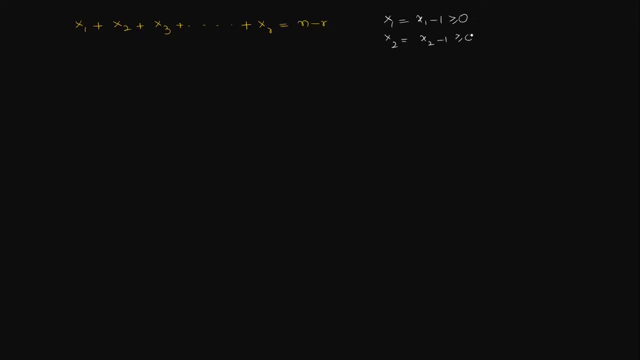 what is x2? Is x2 minus 1, this is also greater than or equal to 0.. Like this, each and every xi is what xi minus 1, which is greater than or equal to 0. So here, x1 is greater than. 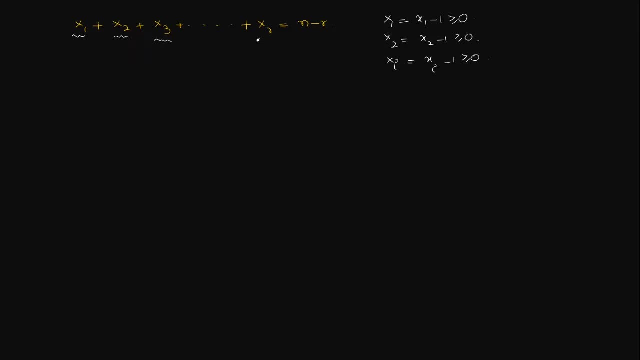 or equal to 0, x2 is greater than or equal to 0, x3 is greater than or equal to 0, xr is greater than or equal to 0. Means these x1, x2, x3, up to so on, xr are what Are non-negative. 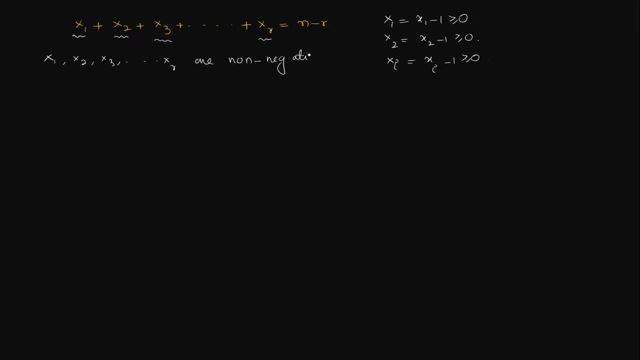 integers, non-negative integers. they are non-negative integers. So, at the end, what we have to find here, We have to find the number of, we have to find the number of non-negative integral solutions. we have to find the number of non-negative integral solutions of this. 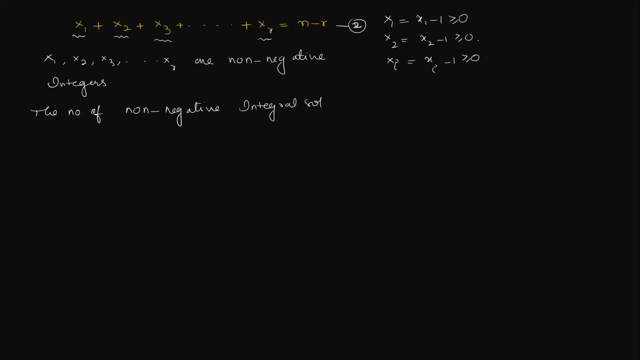 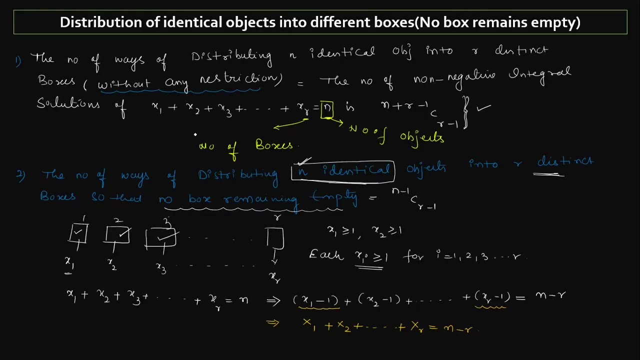 equation. say number 1 or number 2, I will say number of non-negative integral solutions of 2.. So already we have the formula for that number of non-negative integral solutions of this. this say x1 plus x2 plus x3 plus, up to so on, xr is equal to n. what is the? 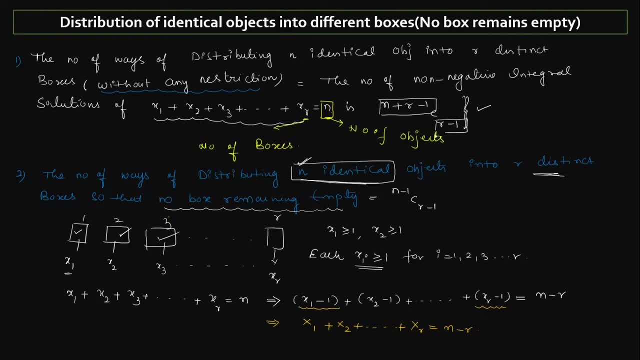 formula: you have n plus r minus 1, cr minus 1.. Have you got this? first Listen? r minus 1 means number of variables, r is what Just now I told you, r is what here Number of boxes and n is what Right hand side number represents the number of objects. 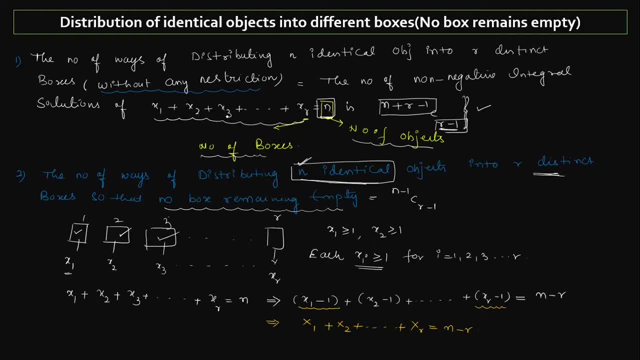 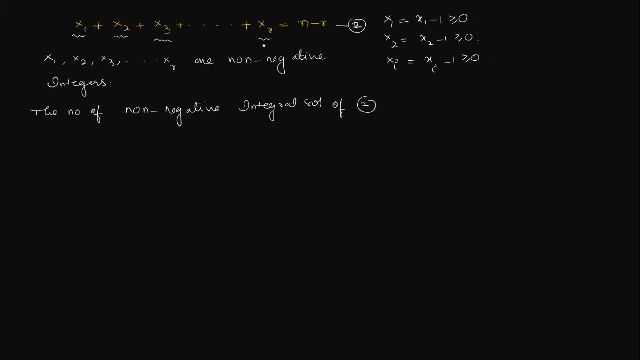 So n right hand side number will be your objects and number of variables will be r. So here is the new equation. Here I got a new equation little bit converted right. Originally equation is different and what we have now is different. But you see how. 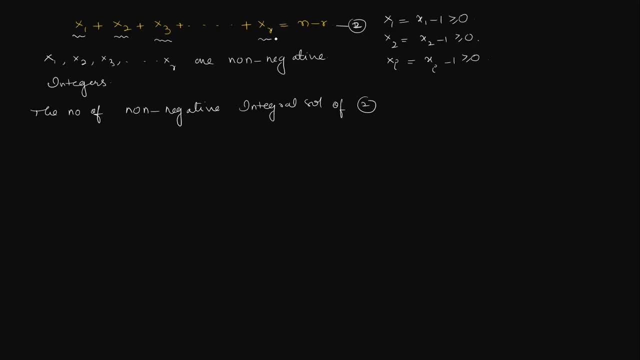 many variables are there? Totally r variables are there. So, therefore, if r variables are there, the answer must be like this: cr minus 1.. And this r minus 1 should be added to what? So this r minus 1 should be added to the. 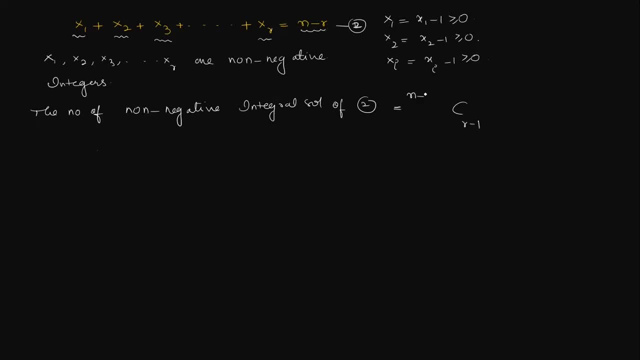 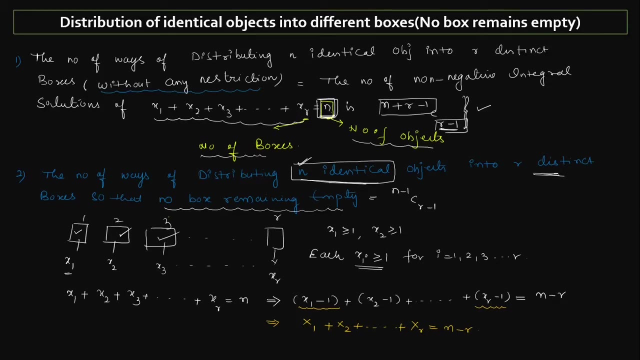 right hand side number right. So here we have n minus r. So n minus r plus r minus 1.. If you want once you can check once again. you check here. n is the right hand side number in the equation. So here we have right hand side is n minus r. There we have the formula. 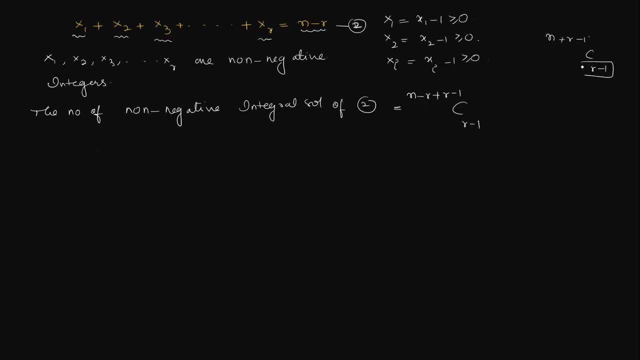 r minus 1, cr minus 1.. These r minus 1, this r minus 1, should be added to the constant which is in the right hand side of the equation. So here in the right hand side of the equation, you have n minus r. So therefore, n minus r plus r minus 1, cr minus 1.. That is number. 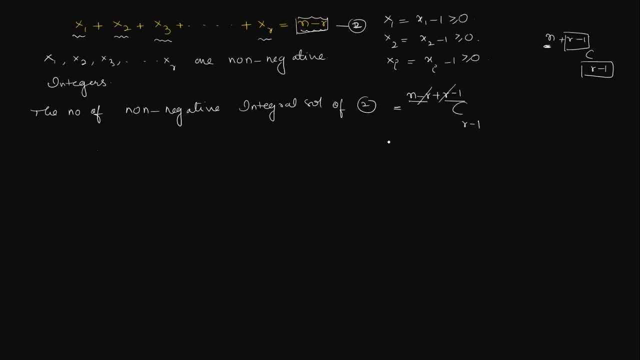 of non-negative integral solutions. So here: plus r, minus r, cancel. So you got here n minus 1, cr minus 1.. So for this second equation, how many solutions are there? That many solutions will be there for this also. 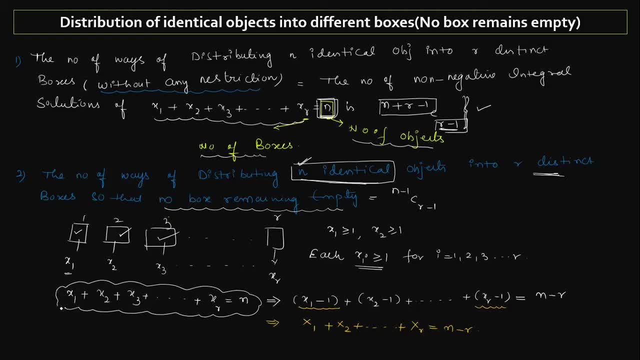 Subtitles by the Amaraorg community. The number of solutions of this equation is same as the number of solutions of this equation. So if you say it has 10 solutions, obviously you are going to have 10 solutions for this. So number of solutions of this equation is same as the number of solutions of this equation. 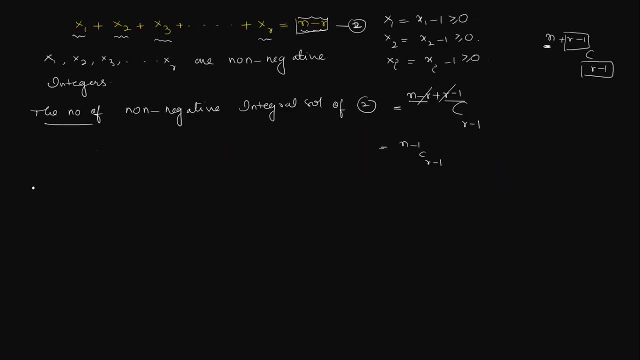 So, therefore, what we can write now, Instead of this, I can write the number of positive integral solutions, Number of positive integral solutions of the original equation. what earlier? what we have, the equation x1 plus x2 plus x3 plus up to so on. xr is equal to n, E is now we got that. 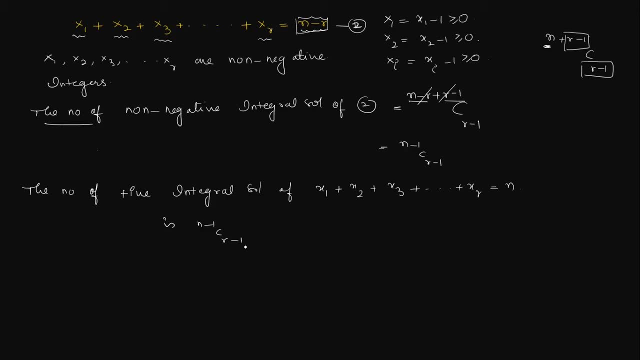 n minus 1, cr minus 1.. So this can be used whenever you want to distribute identical objects into the boxes so that every box contains minimum one object. In that case you can use this formula: n minus 1, cr minus 1, which is nothing but number of objects, the number of identical. 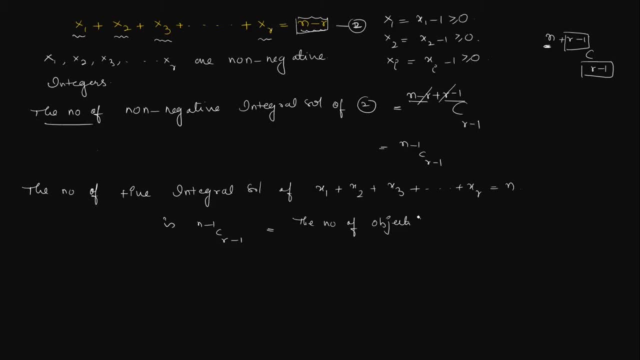 objects. actually, I am writing simply object: the number of objects minus 1, c. the number of boxes. the number of boxes minus 1.. Number of objects minus 1, c. number of boxes minus 1.. So, for example, how many ways, if I ask you a simple question, simple basic question on this, how many ways? 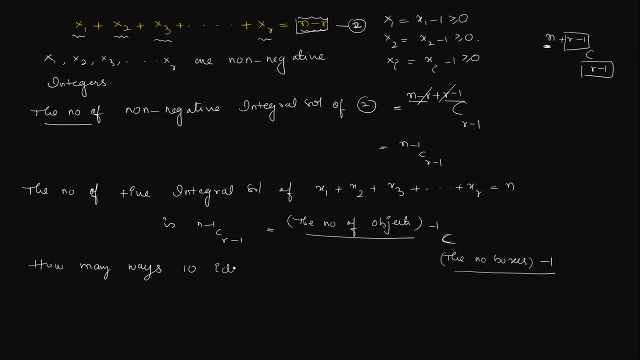 10 identical toys. 10 identical toys can be distributed among can be distributed among 4 children so that each child will get at least one toy. Each child will get at least one toy. So this is nothing but the number of positive, integral solutions, of what 4 children? So you can say: 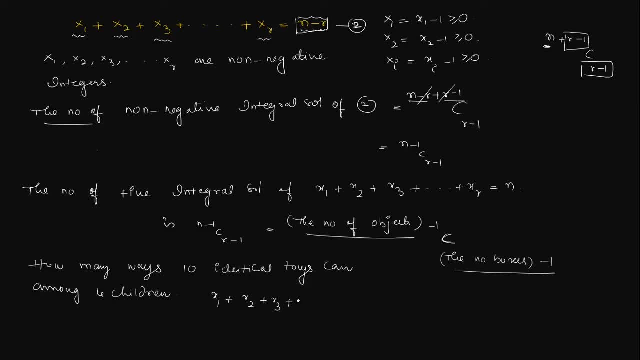 x1 plus x2 plus x3 plus x4. So for first child he will get x1 toys and second child will get x2 toys, third child will get x3 toys and fourth child will get x4 toys. The total number of toys is equals to n. 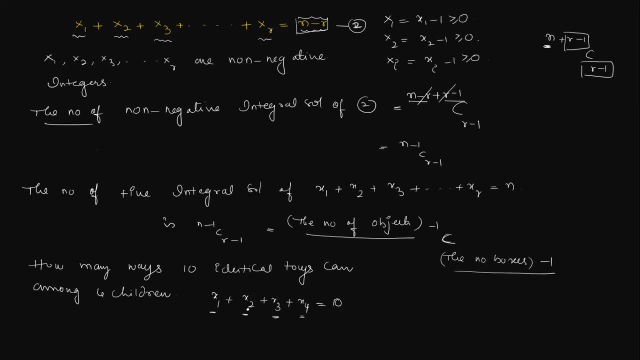 So, indirectly, what is the question is the number of positive integral solutions of this equation. What is the formula we have? The number of objects is 10 minus 1, c number of boxes or number of, is here number of children, right? so four minus one, which is nine c three. you can calculate this.